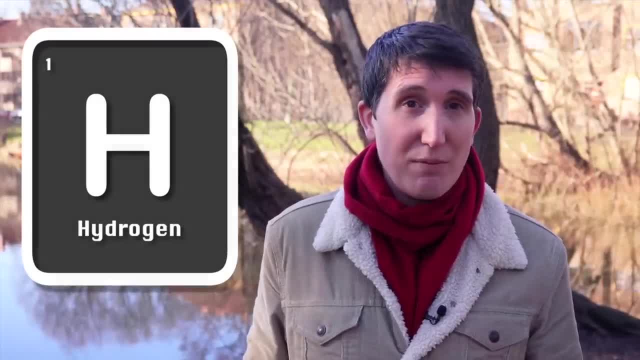 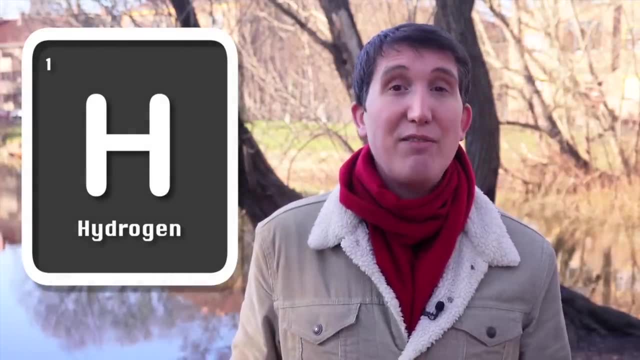 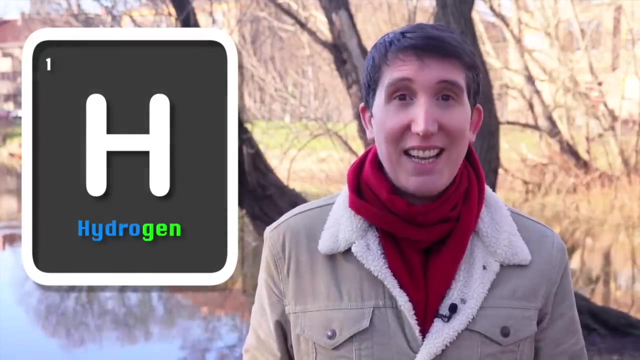 here, because it is one of the elements we're perhaps best acquainted with, but whose name we may never have actually stopped to think about. Hydrogen breaks down into the greek for water, hydro, and the greek for to form or to generate gen. That is the same gen that gives us generate. 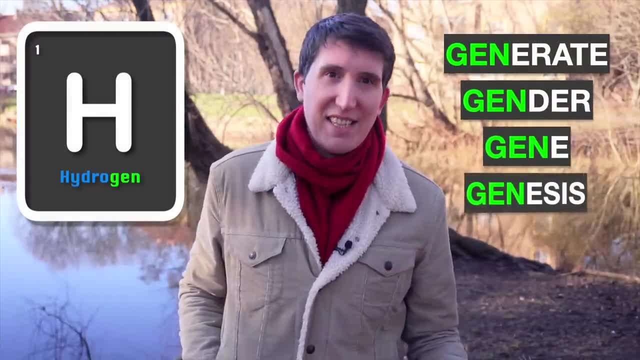 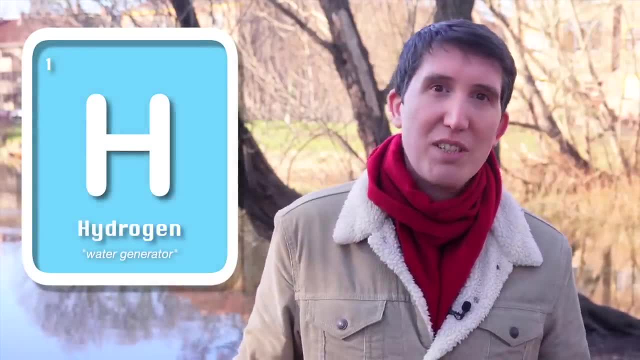 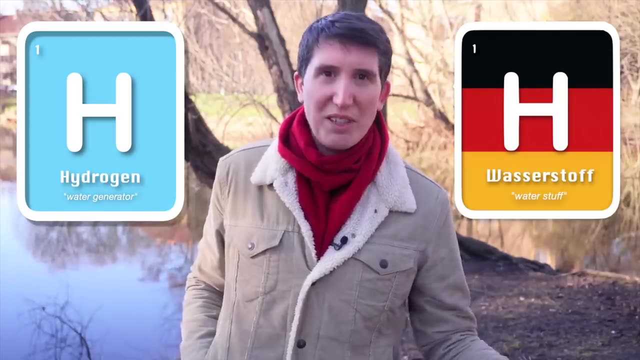 but also gender gene genesis and generous. So why is hydrogen called? That's because it's a name. you need to generate water. In fact, here in Germany, where I'm standing right now, it's called Wasserstoff, which means water stuff or, you know, water material. The other element of water is 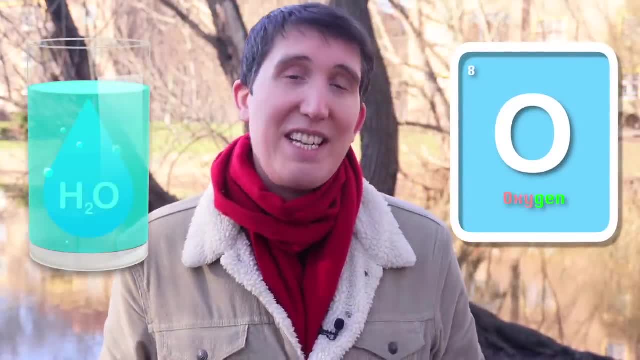 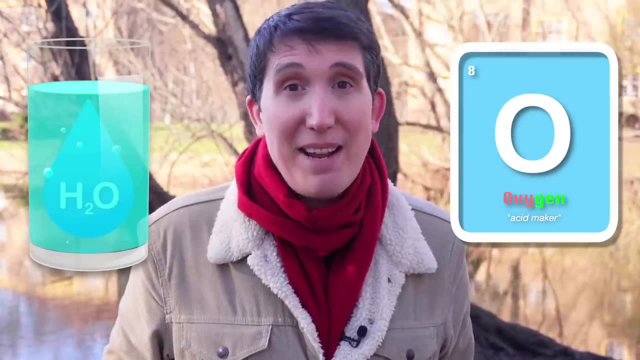 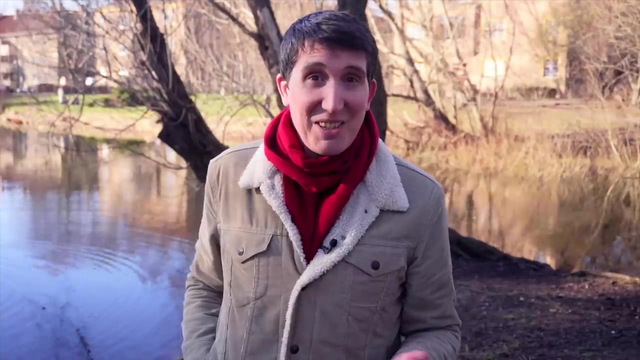 oxygen and there's that gen again. This time the oxy means acid, because it was originally called that under the. it turns out false belief that you needed it to make an acid, So the name's actually misleading. But it could be worse. The scientists who discovered it in the 1700s originally named it deflogisticated. 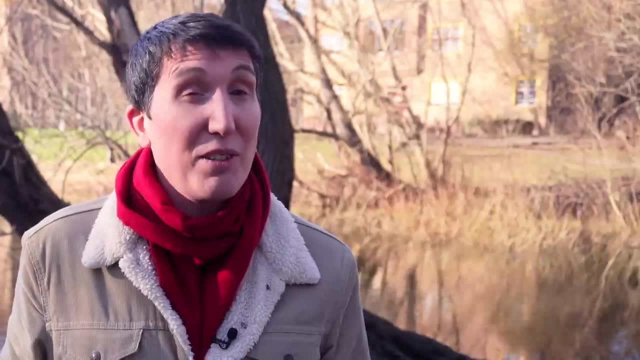 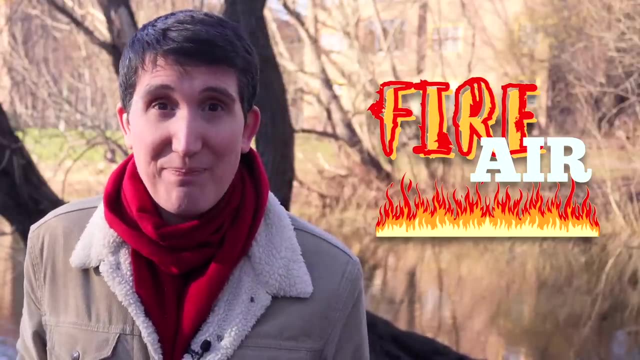 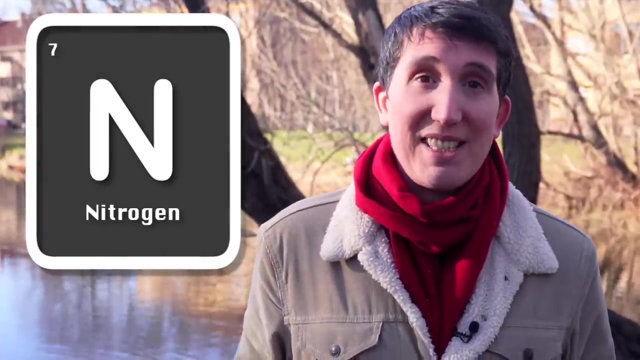 air, So thank god that didn't stick. They also called it fire air, though, which is actually much cooler. Anyway, let's generate another of these gen elements, Nitrogen. it's so called because of its presence in nitre, which is a salt Away from the 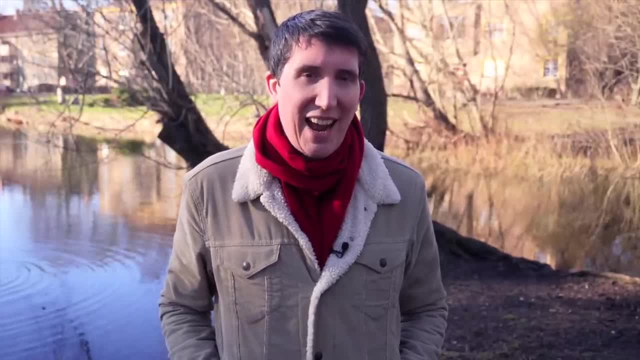 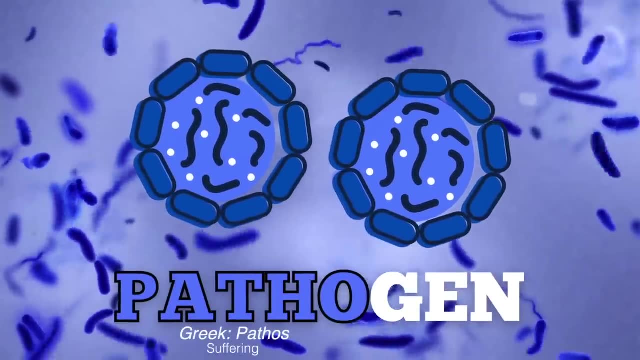 period of time we made these experiment. we're talking about our planet and we're going to table. you can actually see the gen suffix in action in carcinogen, something that generates cancer, or pathogen, something that generates a disease or suffering. actually, I wish I hadn't gone there. that was a bit bleak, wasn't it so? 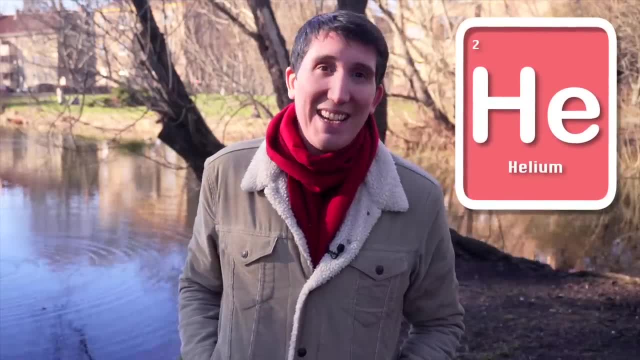 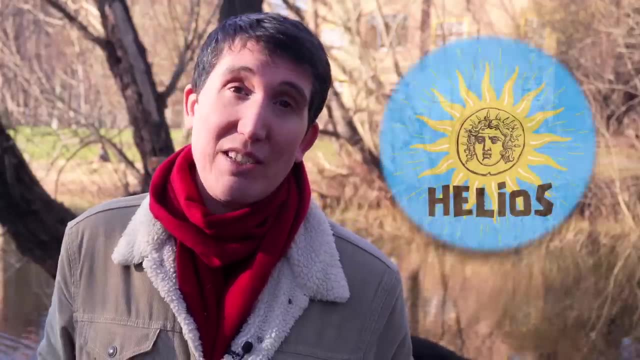 let's lighten things up again with helium. it's also at the top of the table, so it is high time that we talk about it. it gets its name from the Greek god of the Sun, Helios. why? because it was first detected in the corona of the Sun. 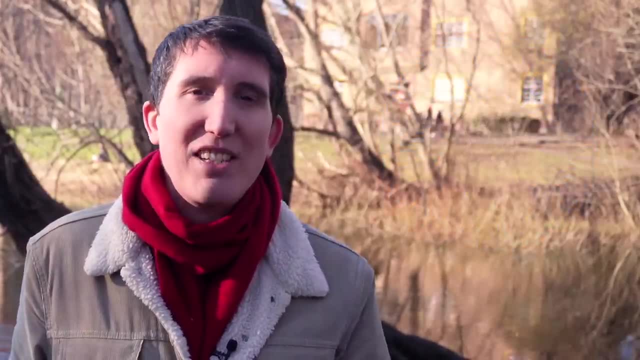 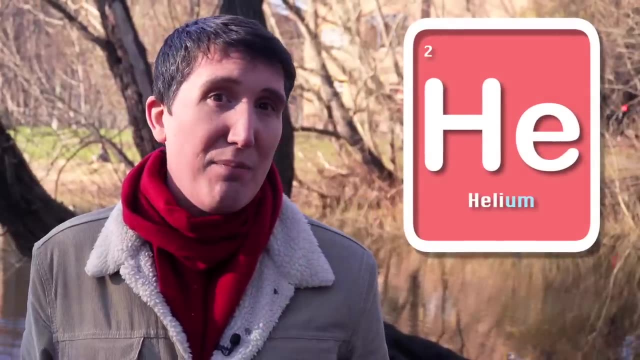 corona itself means crown, and it's the bit you see surrounding the Sun when there's an eclipse. it's that shiny aura. the um at the end of helium is something that we are going to encounter a lot going forward. so let's take a moment to. 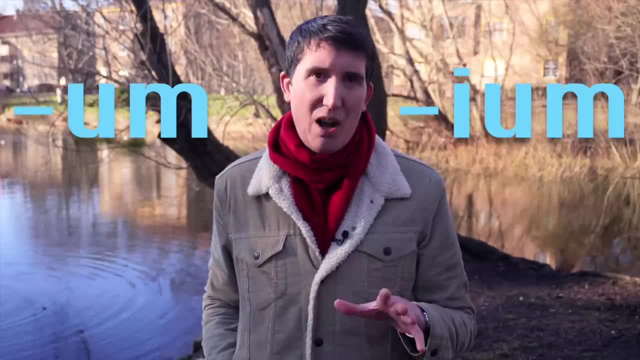 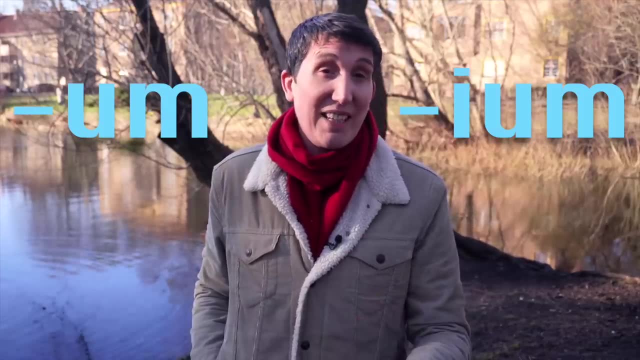 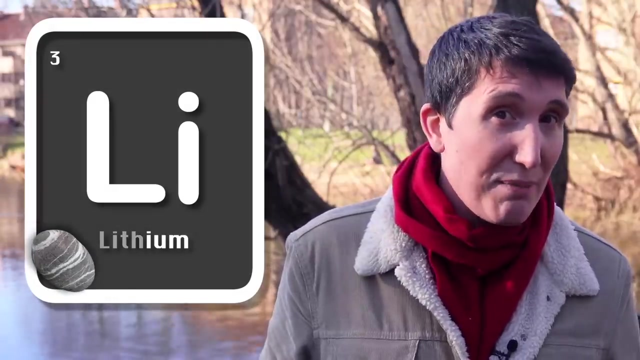 look at it. so both um and eum are just suffixes used to turn something into a substance, etymologically speaking, or specifically into an element. for example, lithium gets its name from the Greek for stone. stone is already a material, but the eum gives us an element. 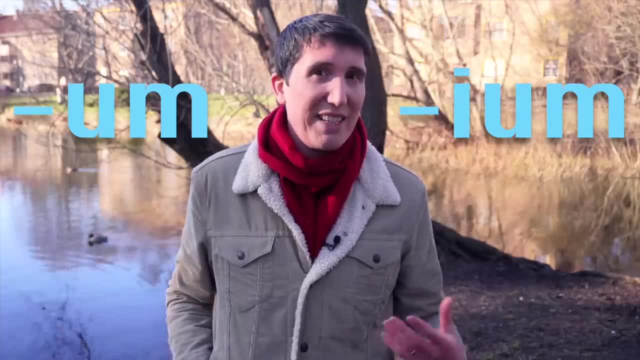 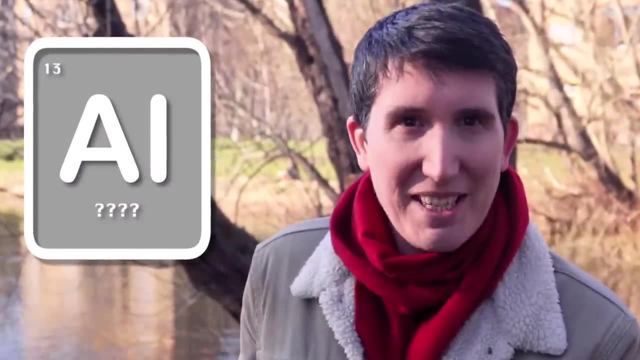 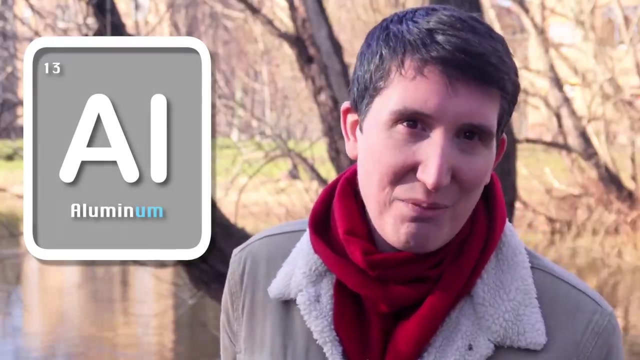 named after it. the fact that there are two similar ways to do this with um and eum is the reason that we have two names for this element here. now I've always called it aluminium, but it also gets called aluminum. now I know you want me to tell you what it is, but I'm not going to tell you what it is because I'm not. 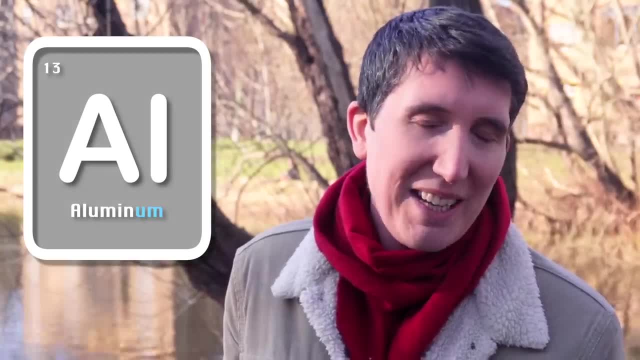 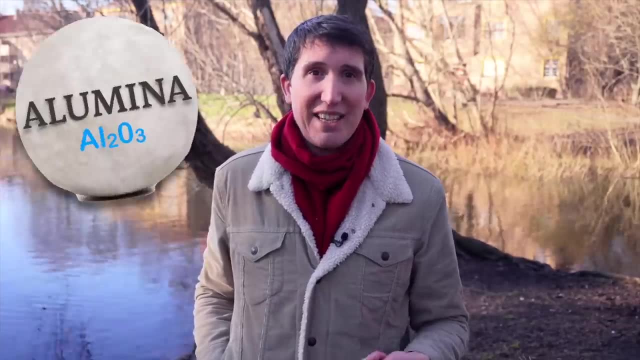 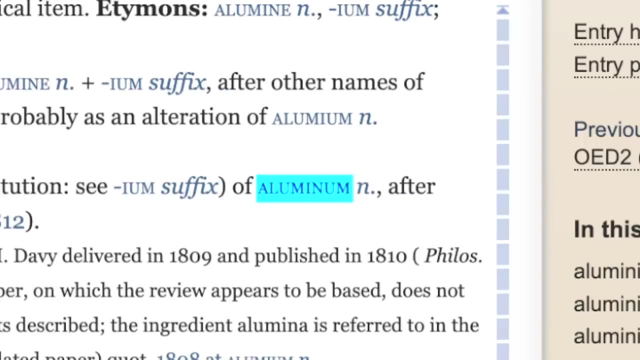 going to tell you which one is right, don't you? well, if only it were so elementary. so aluminium is recorded first as the name for the element you get from alumina. that was in 1811, but then aluminum is seen being used in 1812. 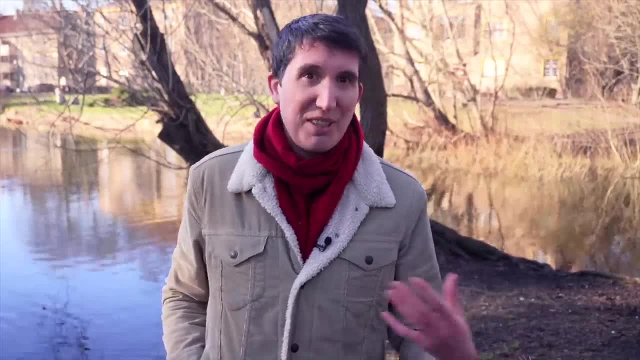 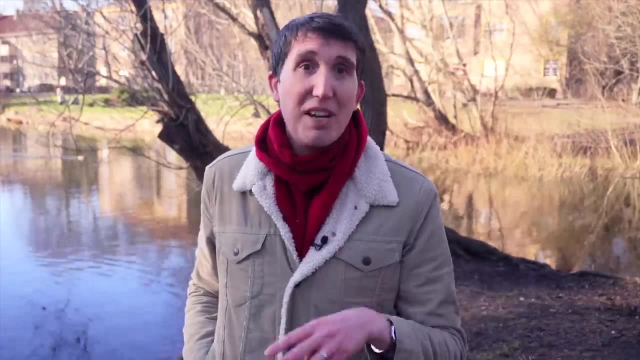 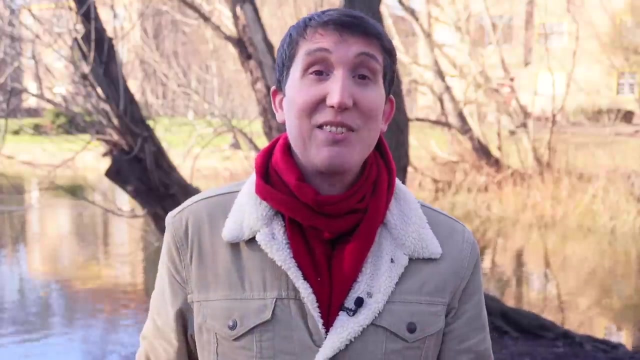 so neither one of them is the long established term and the other one an abominable mispronunciation. they are both good. well, in fact, there was a third option- aluminum- but let's just leave that one buried safely in the ground. instead, let's look at some more of the big hitters from 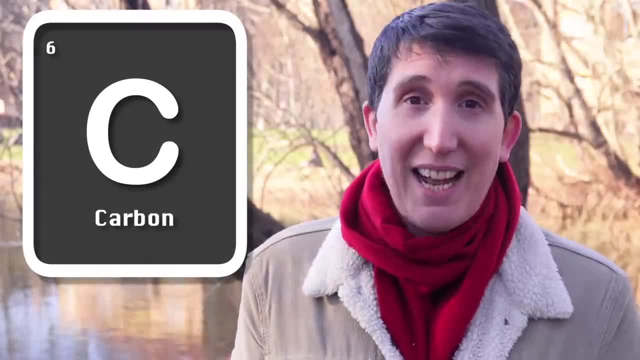 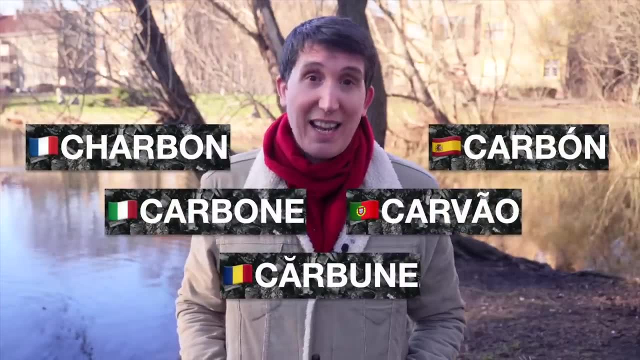 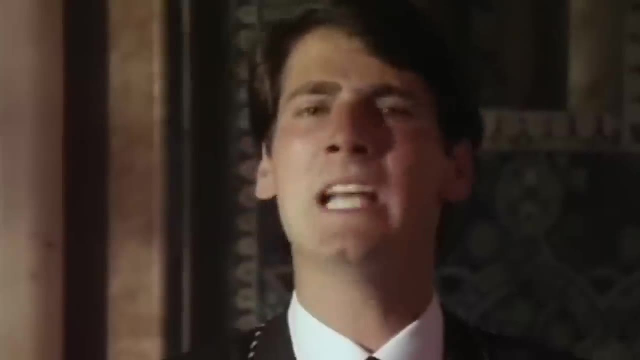 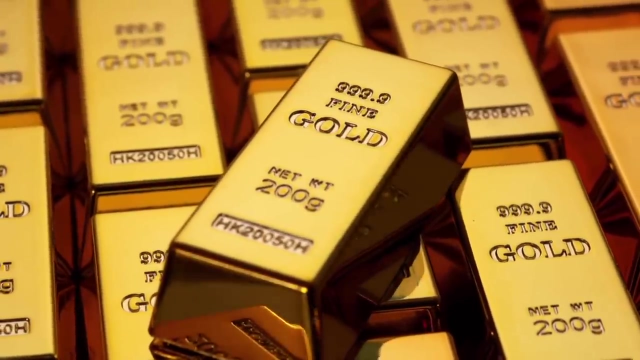 the periodic table. so carbon gets its name from the Latin for coal. coal itself is composed mostly of carbon, and today the words for coal in the Latin languages are something along the lines of carbon. next up is gold. gold is a very old word. we've been calling it something along those lines for as long. 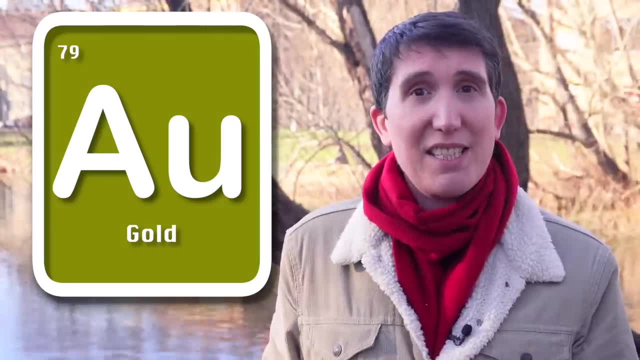 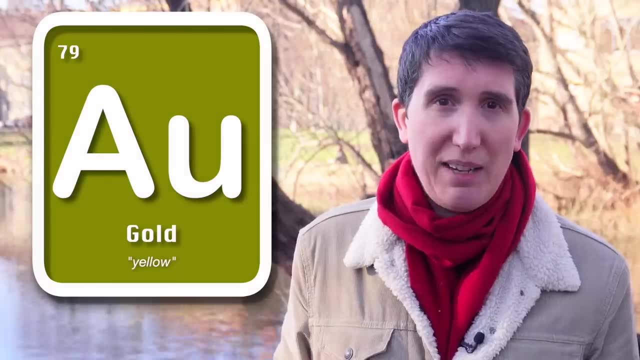 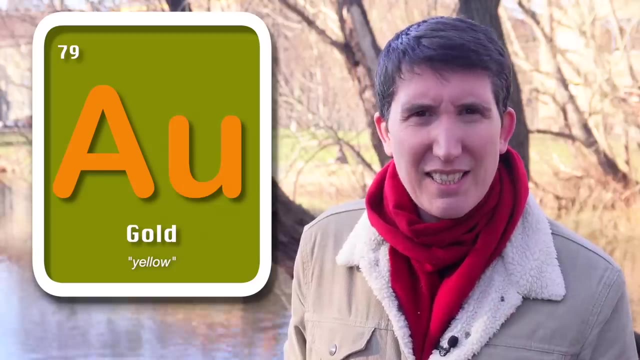 as we can trace the Germanic languages back, but it's thought that its ultimate route is in Proto-Indo-European hila, meaning yellow. but hang on a second. what's going on here? its symbol is a u. now neither of those letters is in the word gold. so what is cracking off here? 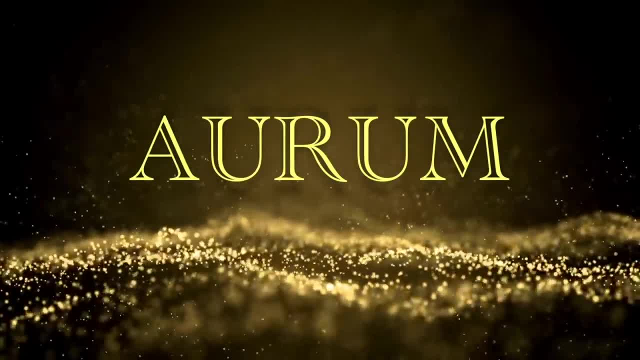 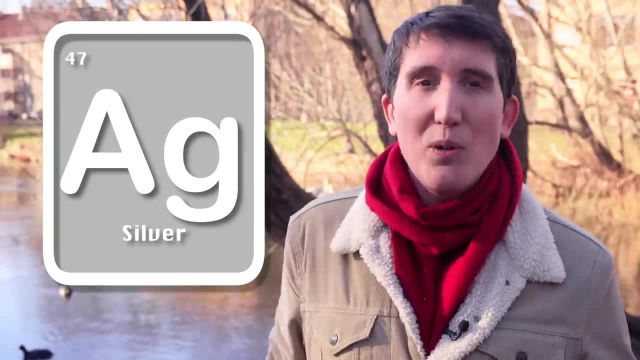 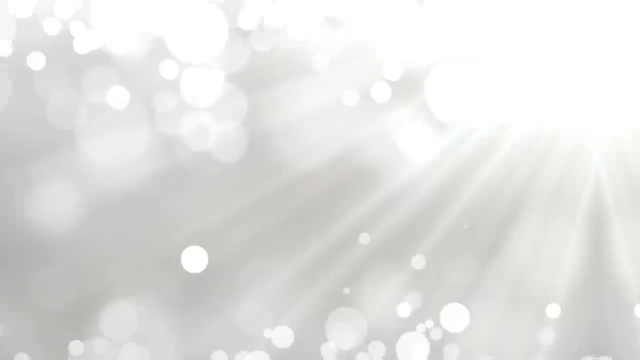 well, that's actually short for the Latin name for gold, Aurum. coming in just behind gold, as it usually does, is silver. now, that's another old Germanic word. but again, what is going on with that chemical symbol? well, AG is short for its Latin name as well: Argentum, in this case from. 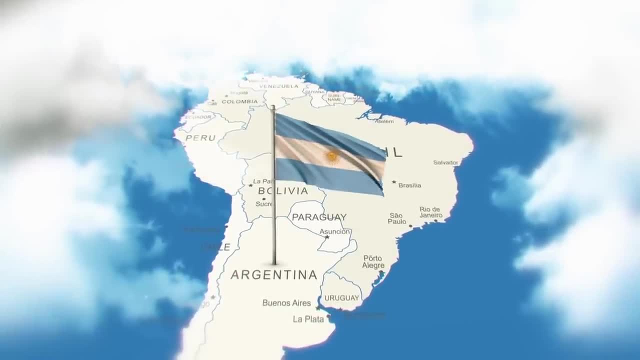 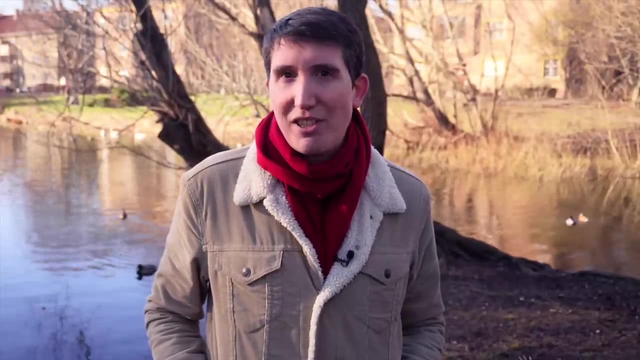 which we actually get the name of the country, Argentina, because when the Spaniards rocked up in the Americas in the 16th and 17th centuries, they were rather excited about the large amounts of the precious metal that they were able to take back with them. they named 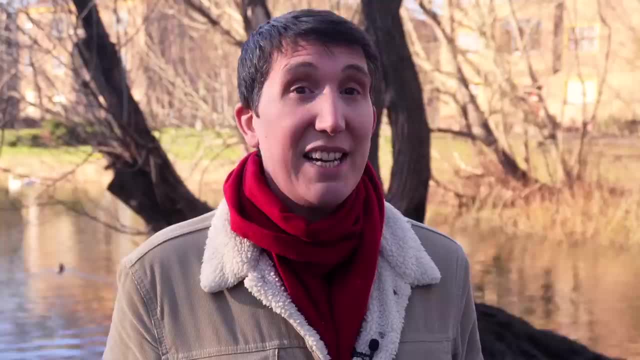 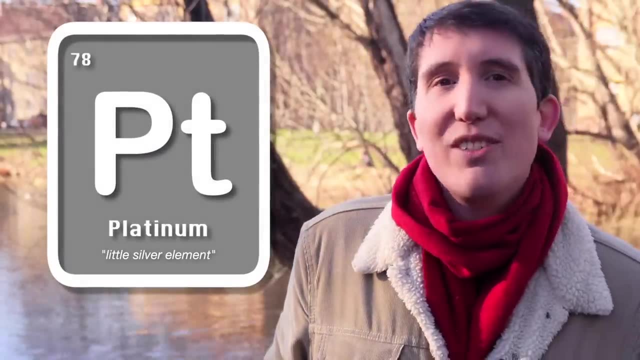 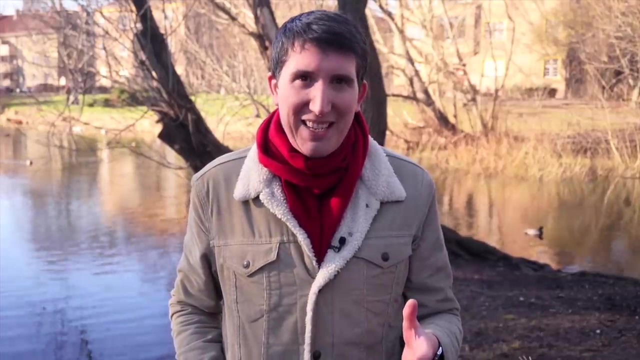 Argentina using the Latin word for silver. but there is an element named after the Spanish word for silver too. platinum comes from the Spanish plata. it means little silver element. platina is a cute little version of platter. basically, the Spaniards thought that platinum was an inferior. 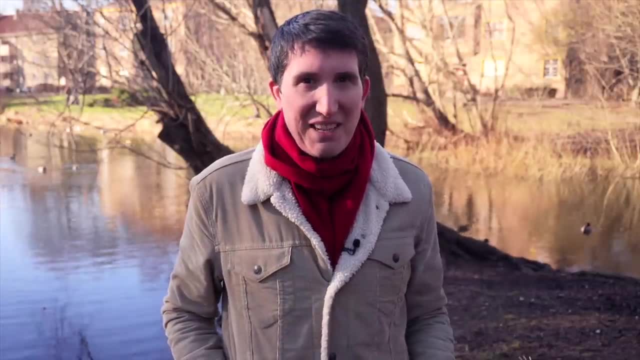 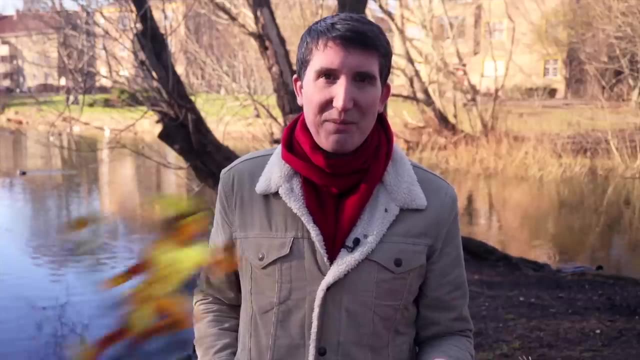 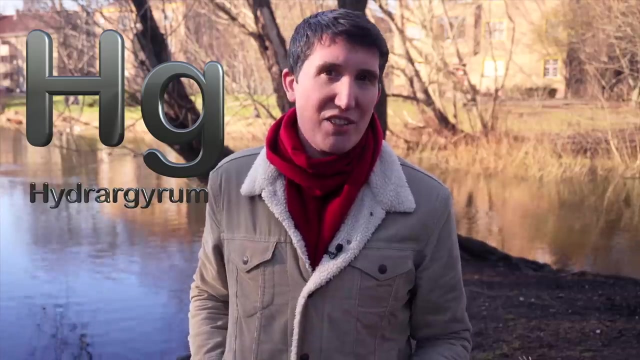 form of silver. how wrong they turned out to be. and there's another element named after silver too. ready Freddy, it's Mercury. so our word Mercury comes from the name of the Roman God, but the chemical symbol is HG, which is short for the Greek Hydragerum. now we've seen the 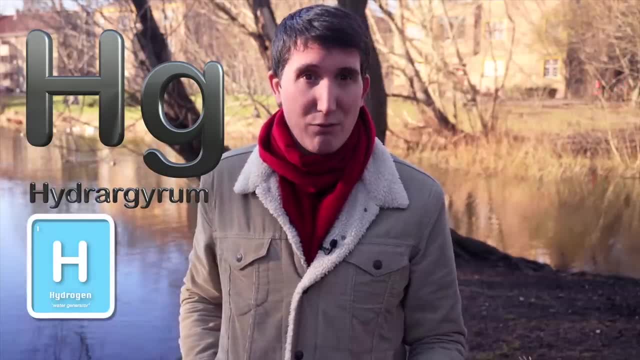 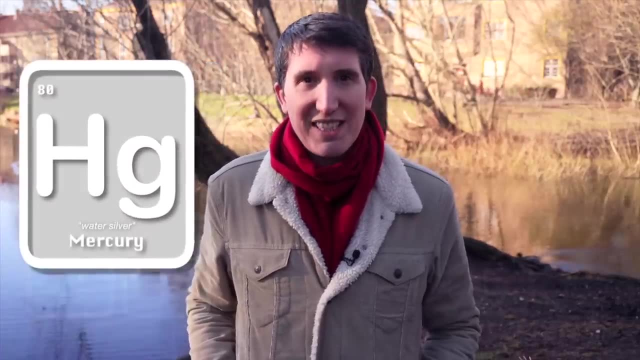 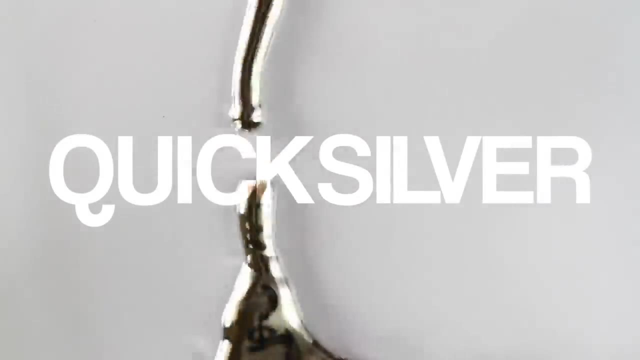 elements of that word before. the Hydra bit is water, like in hydrogen, and the Argerum is silver. Hydragerum means water silver. in fact, Mercury used to be called in English quick silver, which means liquid silver, because that's basically what it looks like. so Argentina may be named after an. 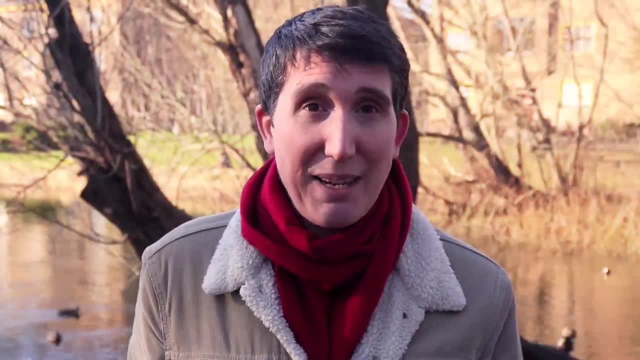 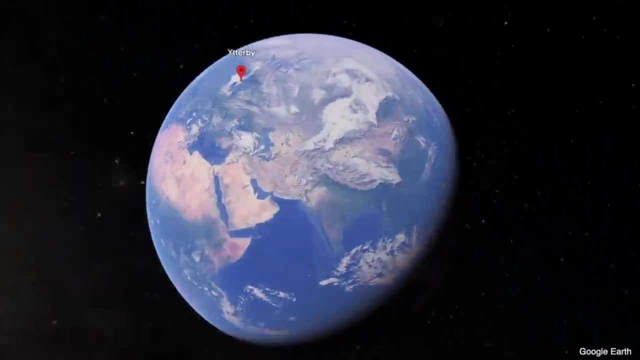 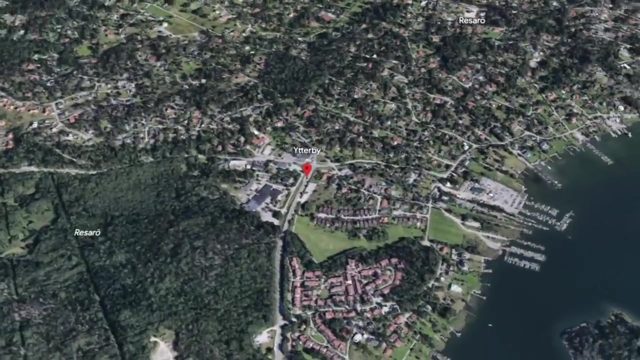 element, but it's actually far more common for elements to be named after places. however, some of them are by no means obvious. one place has more elements named after it than any other, and I'm willing to bet that you've never even heard of it. it's this place just outside of the Swedish capital. 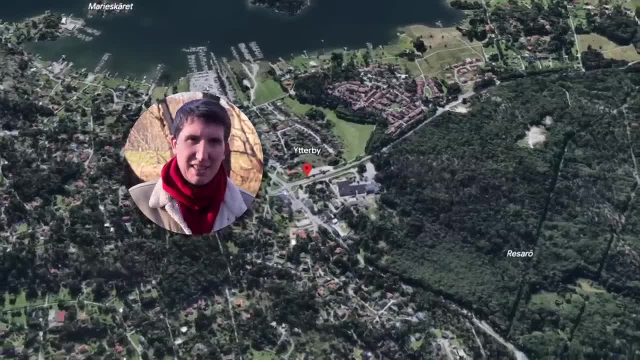 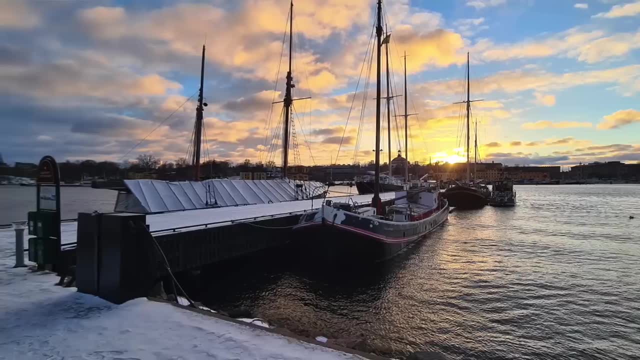 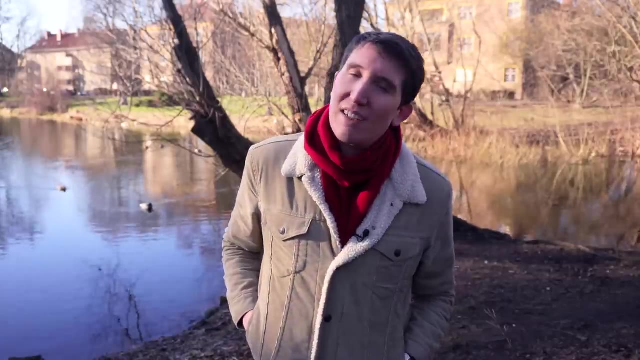 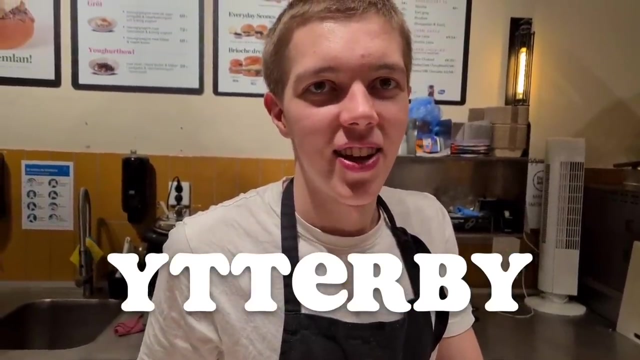 now, I had no idea how to pronounce this, is it it to be absolutely no clue, but I did happen to be in Stockholm the other day, so I took the opportunity to ask a Swede and after pouring me a lovely coffee, barista Isaac kindly obliged. how's it pronounced? and again for me, thank you so much. 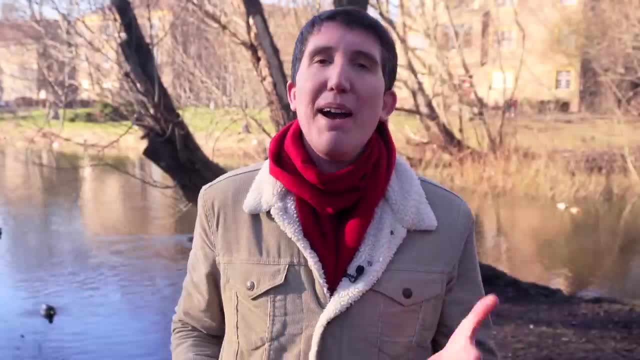 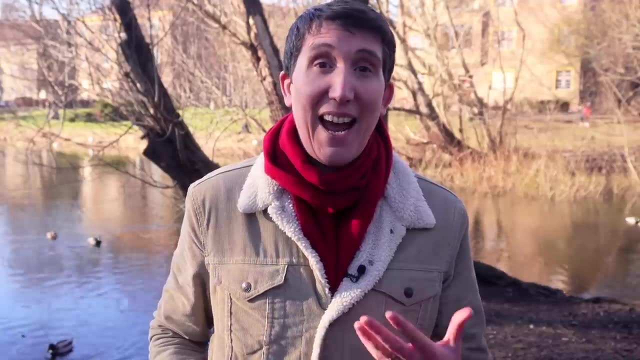 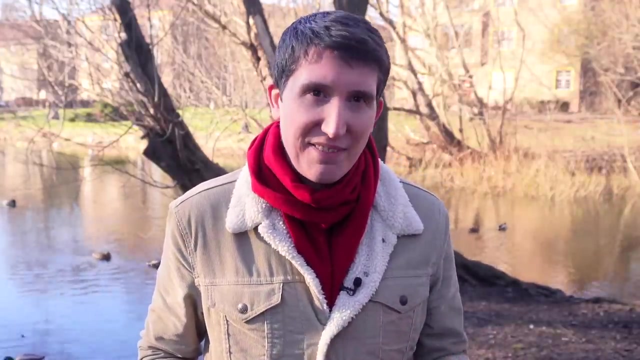 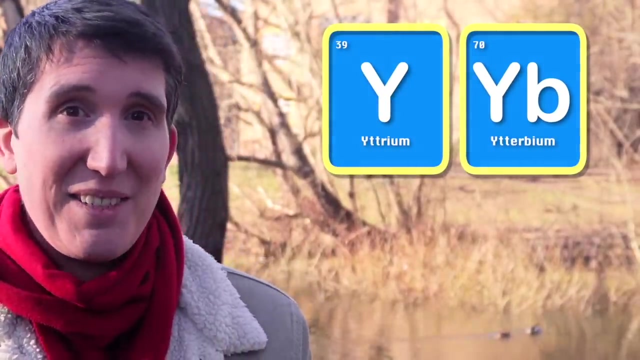 still can't get it right anyway. back in 1789, the first rare Earth metal compound was found in a lump of rock taken from a mine at it, and since then a whole host of brand new elements have been identified there, among them yttrium and ytterbium, which are both quite obviously named after the. 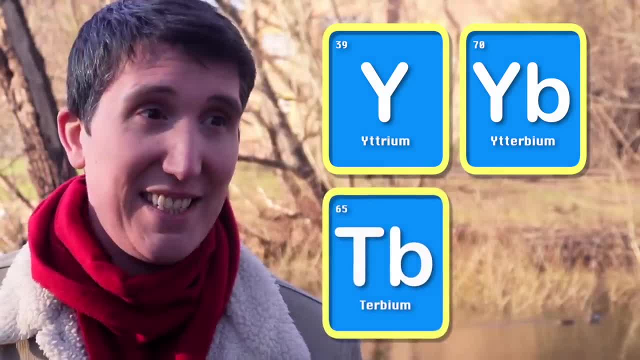 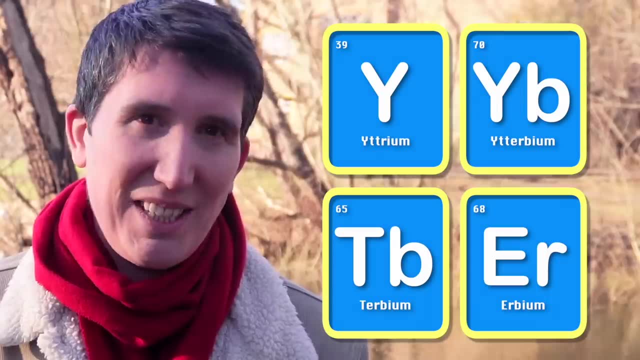 place, but so also is terbium, and indeed So a whole four elements are named after that one tiny town on the Baltic coast. Zero points for creativity, though. I bet they wanted to call the next one just Bium, but they didn't. 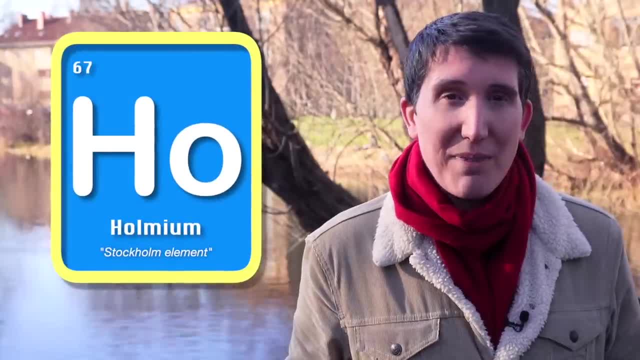 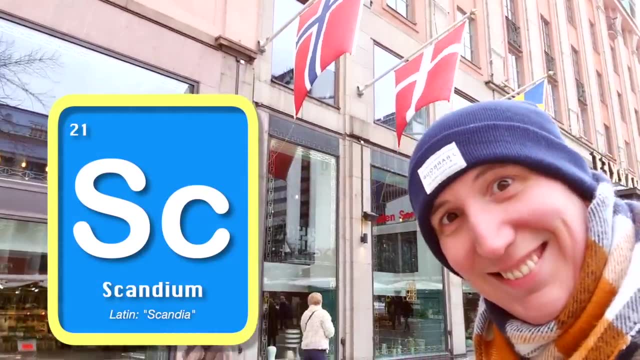 But other elements were found there. One of them was named Holmium, after nearby Stockholm, Another one was called Scandium, from Scandia, the Latin name for Scandinavia, And there's also Thulium, which comes from Thul, an ancient Greek and Latin word. 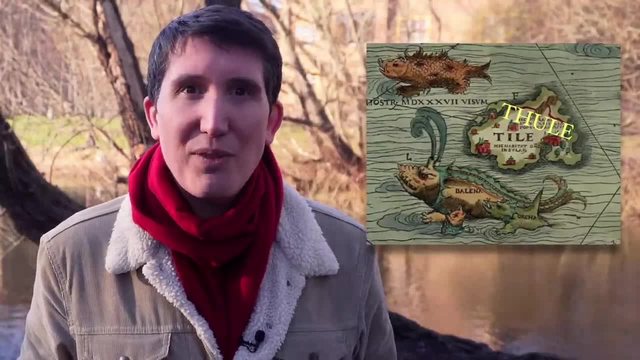 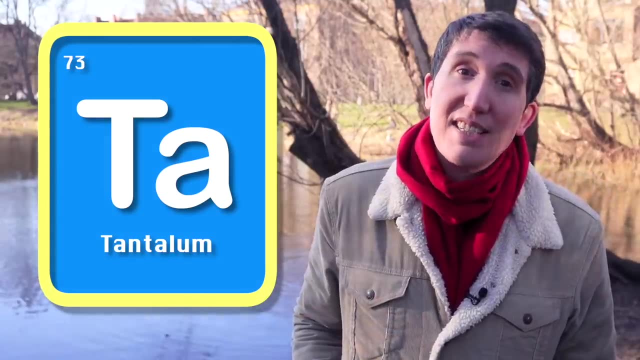 for what they believed to be the most northerly region of the world. Tantalum was also found at and, in a bit of a sidestep, was named after the Greek mythological character Tantalus. Now, that poor fellow was doomed to an eternity of hunger and thirst. 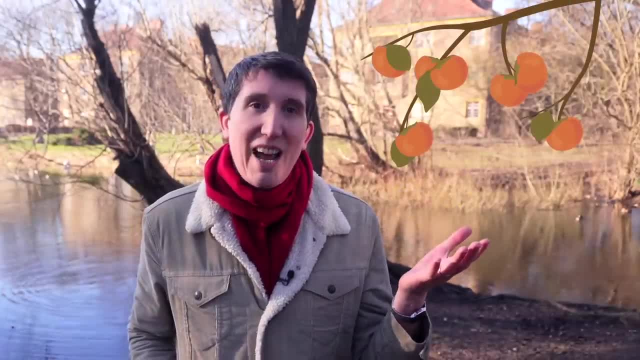 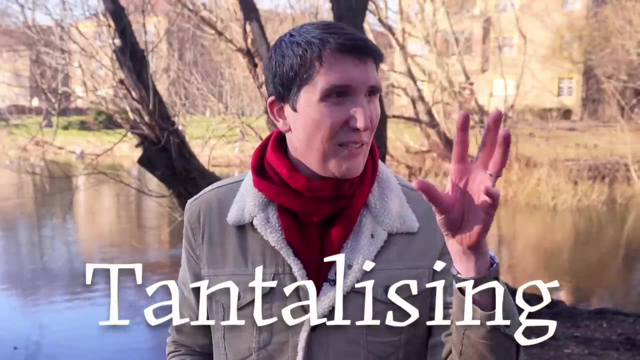 standing under a tree of fruit that he couldn't reach and in a pool of water that he couldn't drink. We get the word tantalum, We get the word tantalising from him to express a desire that is, you know, just beyond our grasp. 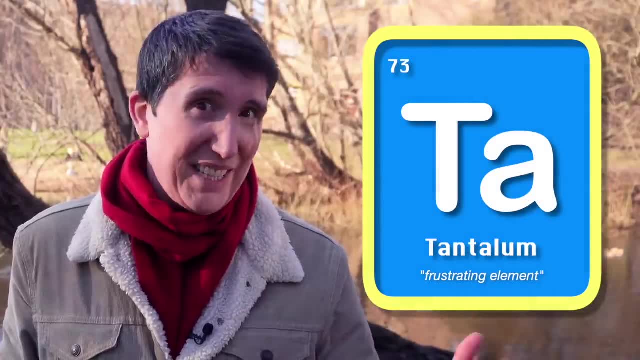 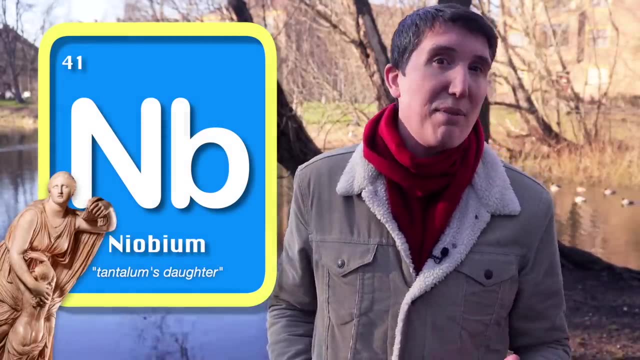 And tantalum is named after him because it's really difficult to separate from its awe. Another element, Niobium, is named after King Tantalus's daughter, Niobe, because tantalum and niobium are always found together. More on Greek mythology to come. 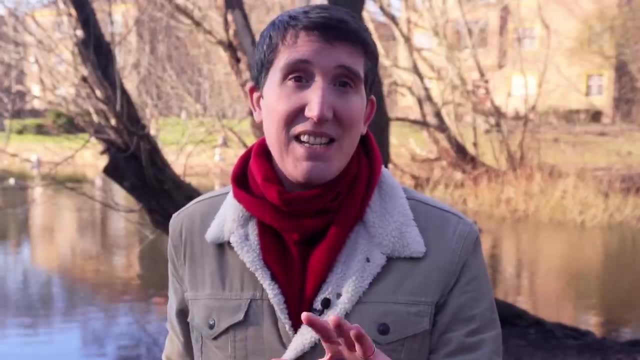 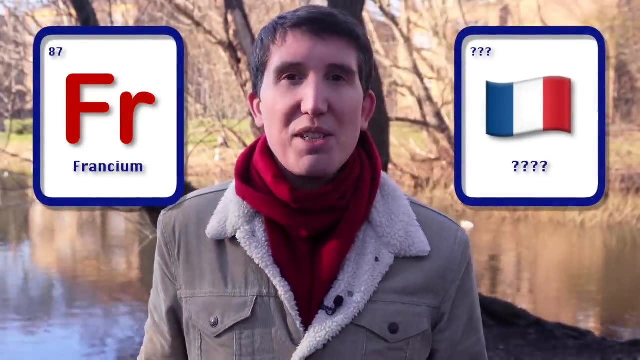 but let's look at some more elements that are named after places. first, Now, France gets two elements named after. We've got Frankium, which is obvious, but also Gallium, which gets its name from the Latin name for France, Gallia. 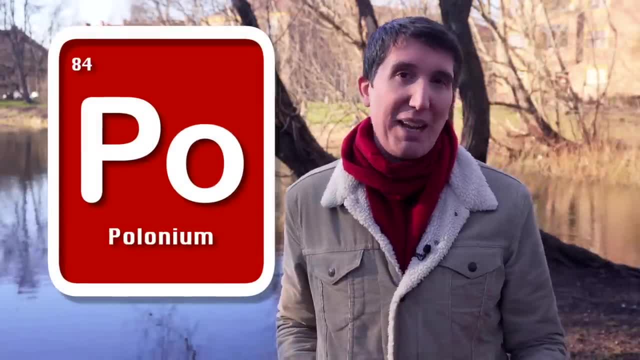 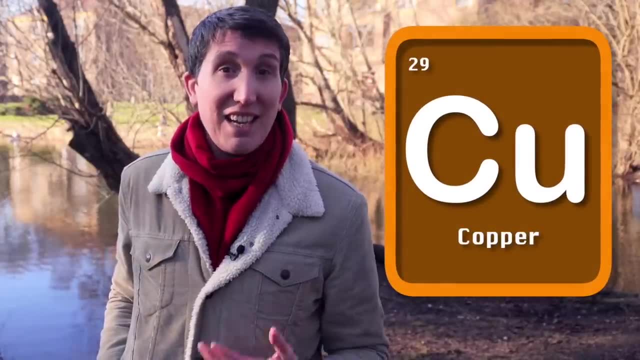 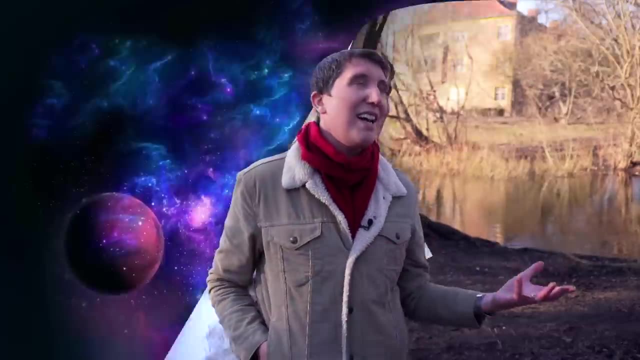 Other elements named after places include Polonium, named after Marie Curie's homeland, which was not France but Poland. Copper is ultimately named after the island of Cyprus, from where the Romans sourced most of theirs, And some other examples are truly out of this world. 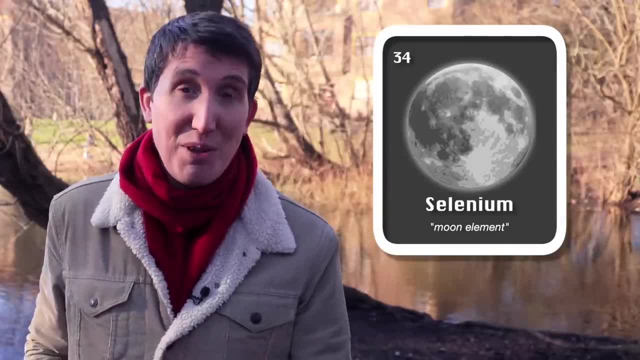 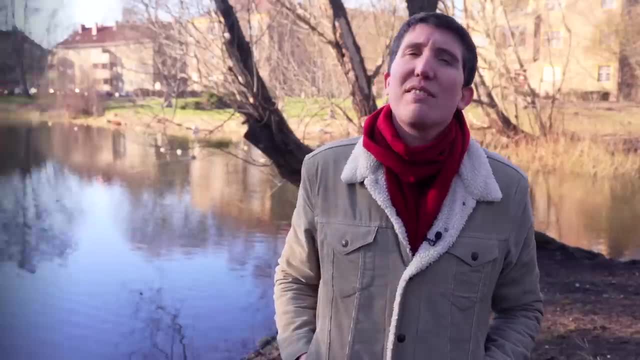 Selenium gets its name from the Greek word, from the Greek word for the moon. Selene And Uranium, Neptunium and Plutonium are all named after planets. There are loads of others named after places too. I'm not going to go through all of them, but you can see them all there. 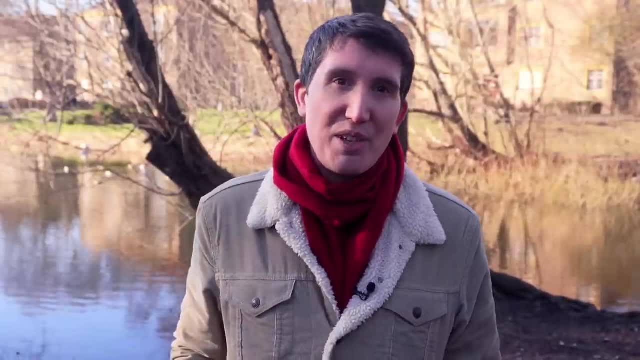 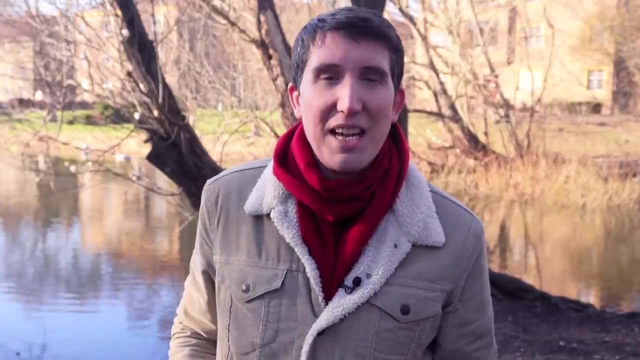 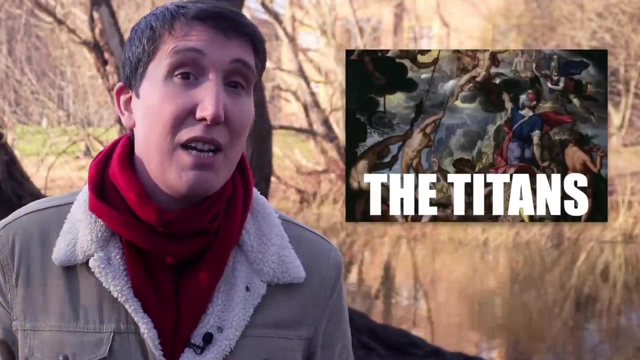 Now the planets Uranus, Neptune and Pluto get their names from Greek and Roman gods, And there are also plenty of mythical figures hidden within the periodic table. Titanium is named after the Titans, the fearsome Greek dead, the deities who preceded the Olympian gods. 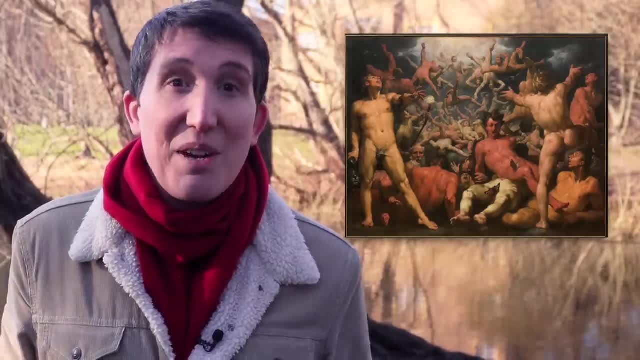 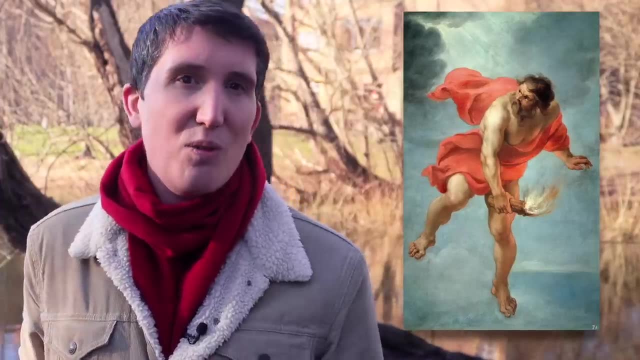 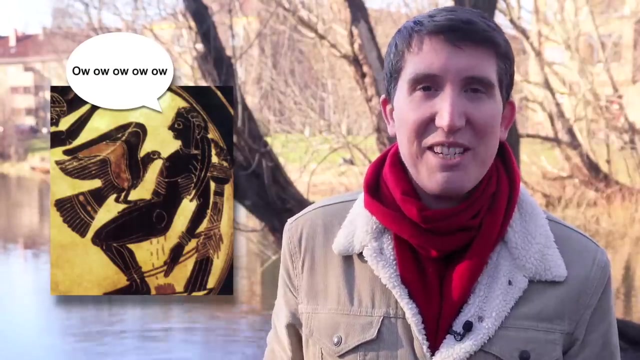 before being banished to the depths of the underworld. Prometheum is named after one of the Titans, in particular Prometheus, who, according to the Greeks, stole fire from the other gods and gave it to humans. He was punished by having an eagle peck out his liver every day for eternity. 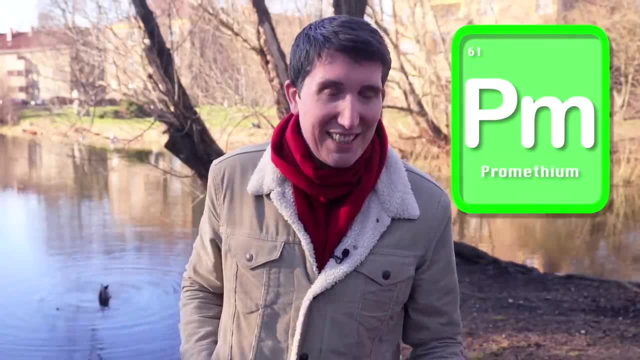 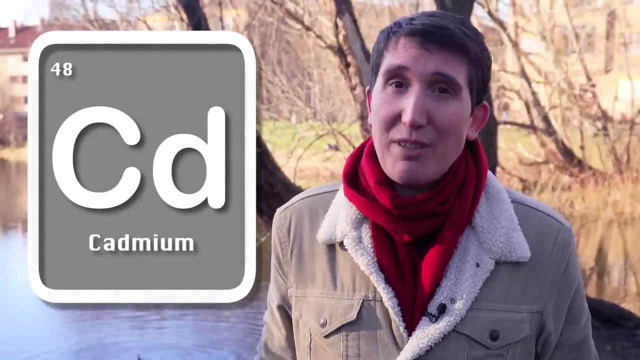 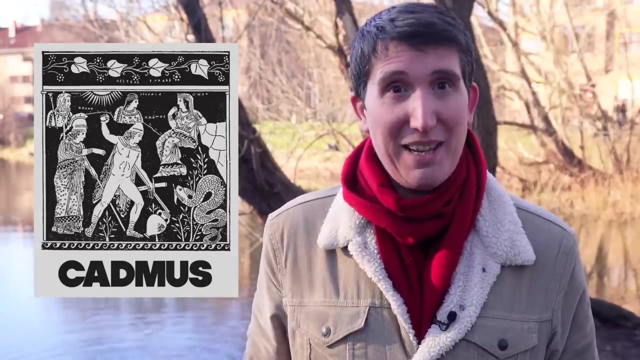 The name of the element is a nod to the excruciating difficulty scientists experienced trying to synthesize. Cadmium gets its name from the Greek mythological king Cadmus, who Greek historian Herodotus claims was responsible for handing the Phoenician alphabet to the Greeks. 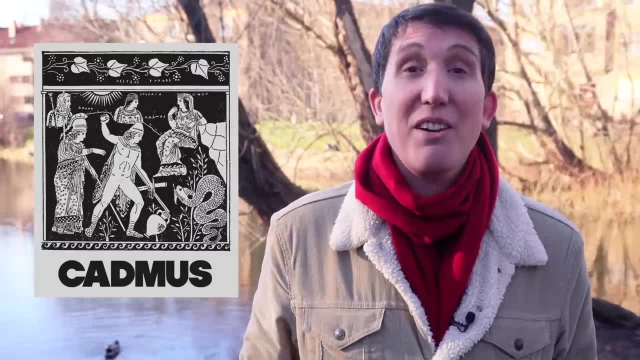 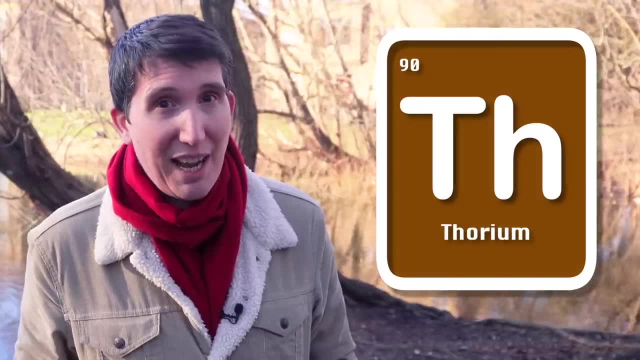 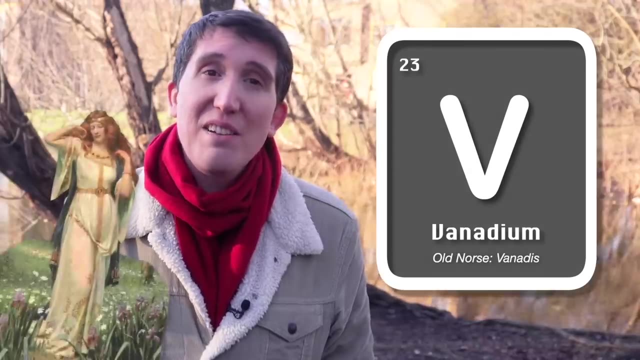 A lovely little crossover fact if you watched my video about the origins of our alphabet, Norse mythology is also represented in the periodic table in the forms of Thorium, named after thunder god, Thor, and Vanadium, which comes from one of the many old Norse names for the goddess Freyja. 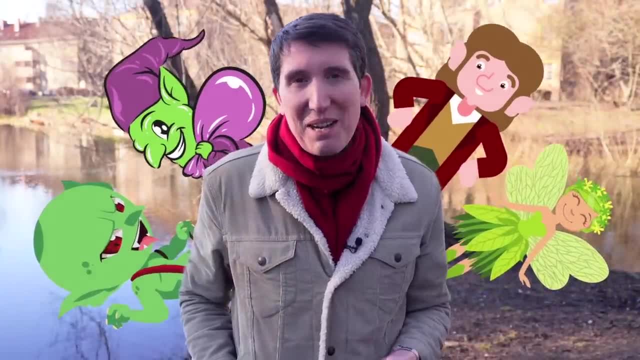 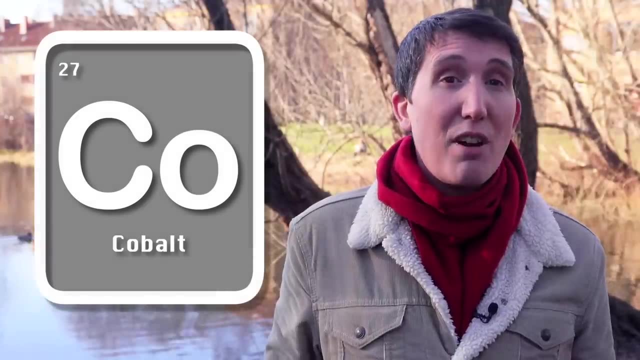 There are also a couple of other mischievous mythical fellows hiding within the table of elements. They're disguised in the forms of cobalt and nickel. Now, cobalt comes from a German word meaning a pixie or a goblin kobold. And nickel is actually a shortening of the German word Kupfernickel. Kupfer means copper, and nickel is another mischievous demon. So Kupfernickel is a sort of copper imp, And nickel gets their impish names because of the ways they confounded the miners who tried to dig them up. 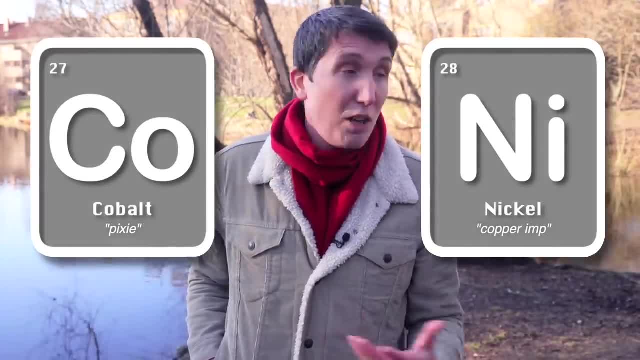 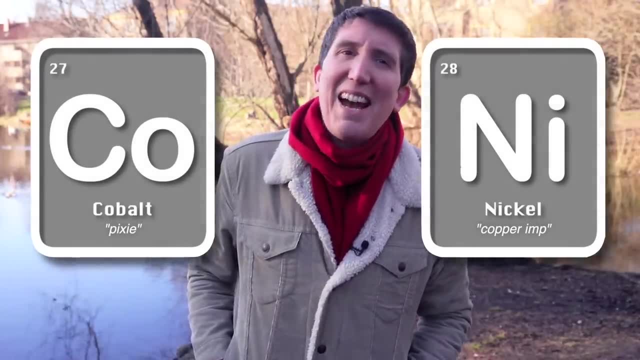 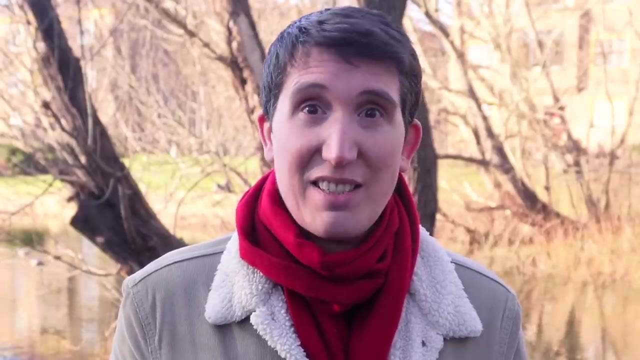 Nickel fooled them into thinking that they were mining. copper and cobalt actually made them ill, or so the miners thought. It was actually probably more likely the arsenic and sulphur that it was mixed in with. Actually, a fair few elements get their names simply from the fact that they are hard to extract. 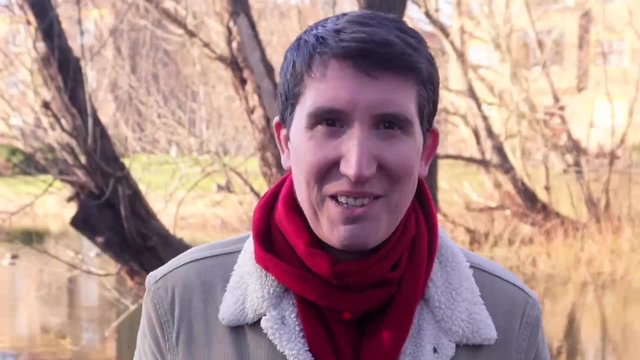 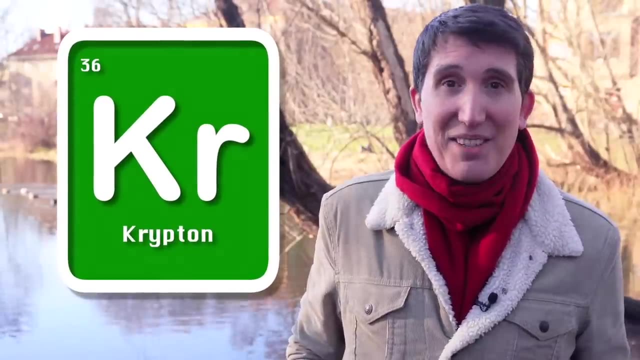 It's as if the scientists were so livid about the trouble that they'd had to go to to isolate or synthesize them that they took it out on the elements themselves. Krypton is not named after Superman's home planet, but the Greek word for hidden. 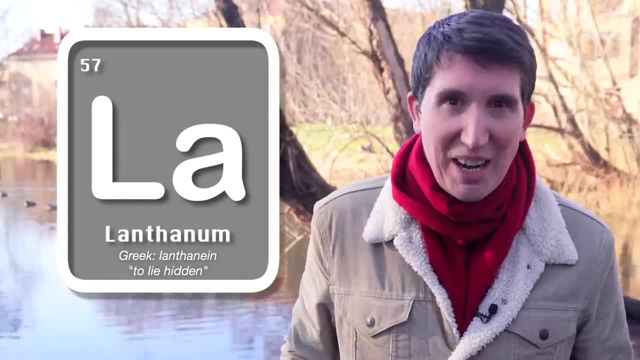 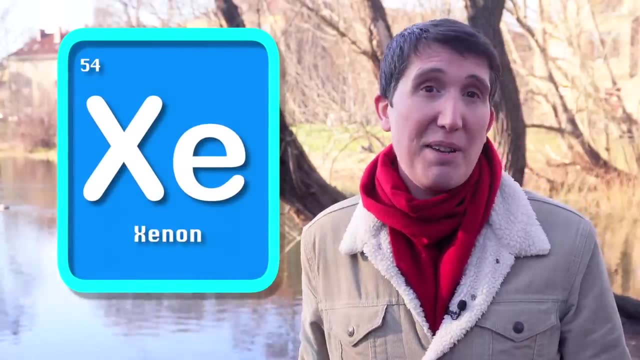 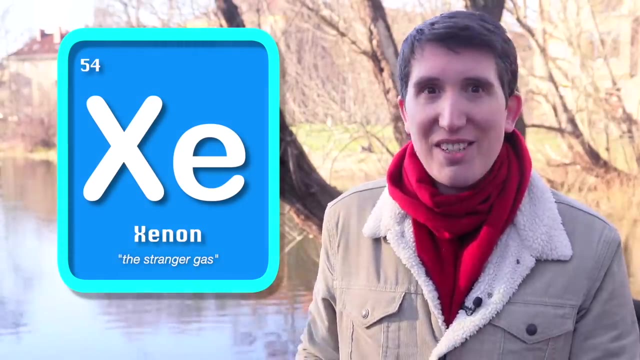 Lanthanum is also named for its shyness, I suppose, and so is dysprosium. Xenon comes from the same root as xenophobia. It's from the Greek for strange or foreign. Xenon gets called the stranger gas. not because it's antisocial, though. 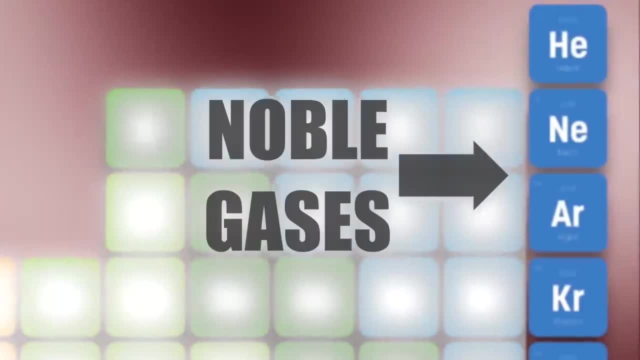 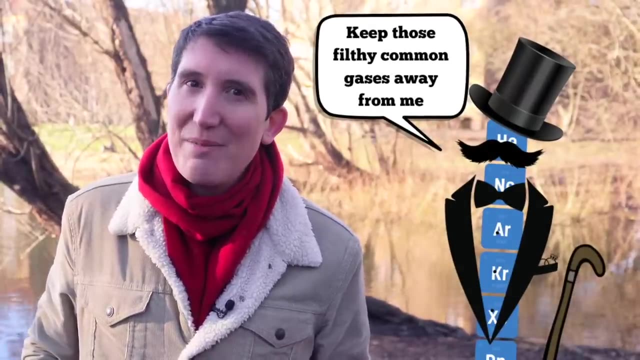 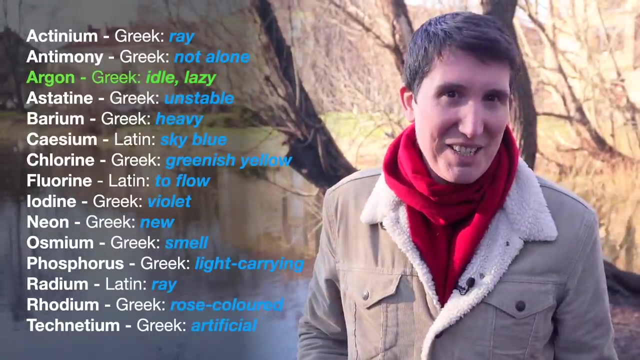 but because it's uncharacteristically reactive For a noble gas. They're called noble because of their reluctance to be associated with other, lesser elements. These elements are also all named after their specific characteristics. My favourite among them is argon, which gets its name from the Greek for lazy. 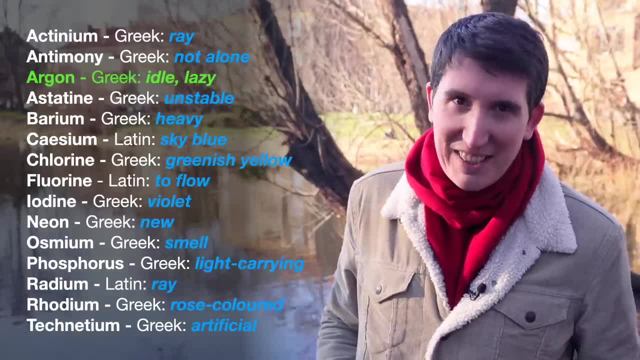 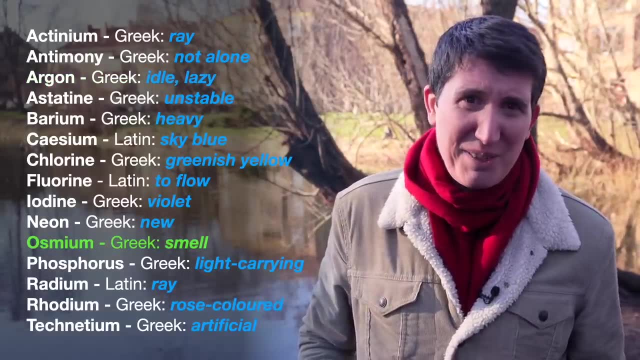 just because it basically can't be arsed to react with anything. And also there's poor old osmium, which gets its name from the Greek for stink because it smells, Or at least the compound the scientist used, Who named it was working with, did. 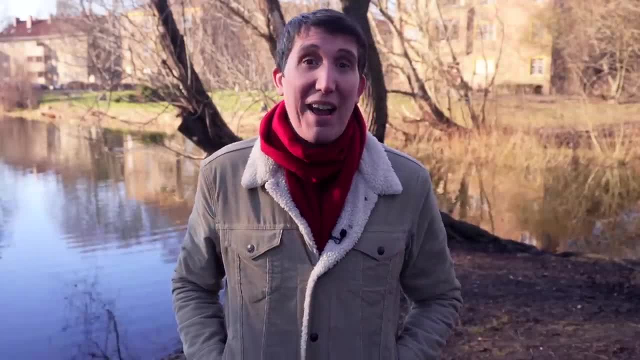 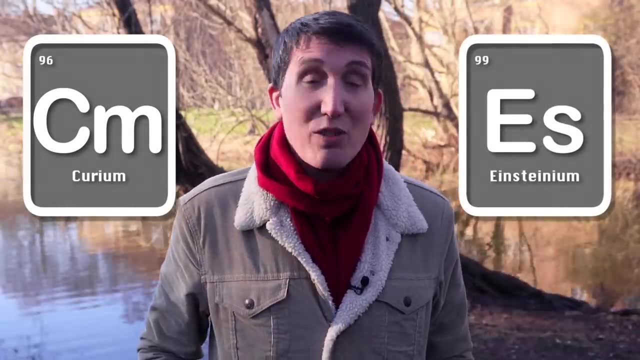 Now, often, scientists themselves end up being immortalised in the names of elements. Curium is named after Pierre and Marie Curie, Einsteinium is well, do I really need to tell you? And there's also nobellium and copernicium. 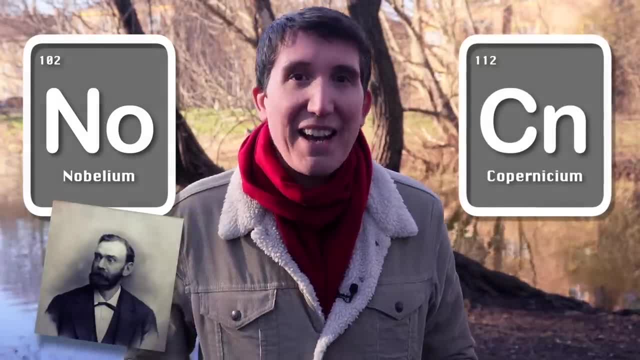 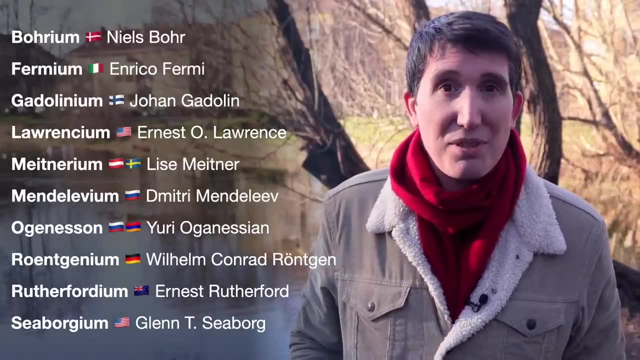 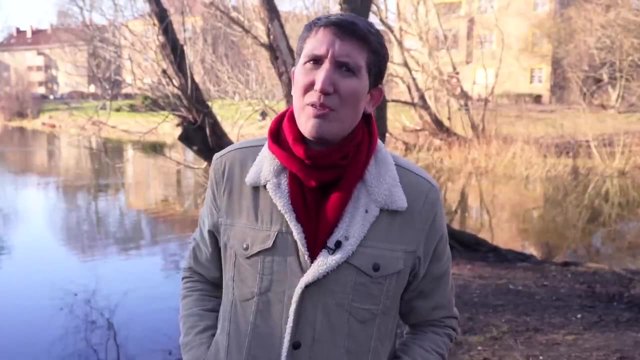 named after Alfred Nobel, of dynamite and Nobel Prize fame and Renaissance brain box, Nicolaus Copernicus. All of these other elements are also named after people too. Some you may have heard of, others maybe not Now. I want to mention some more of the confusing name-chemical-symbol combinations. 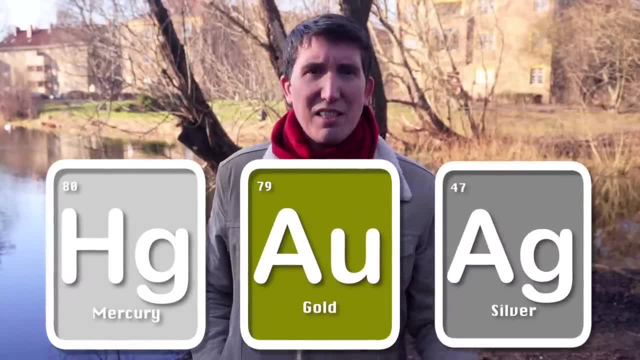 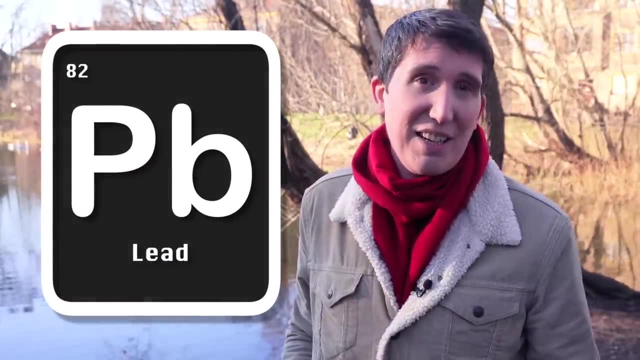 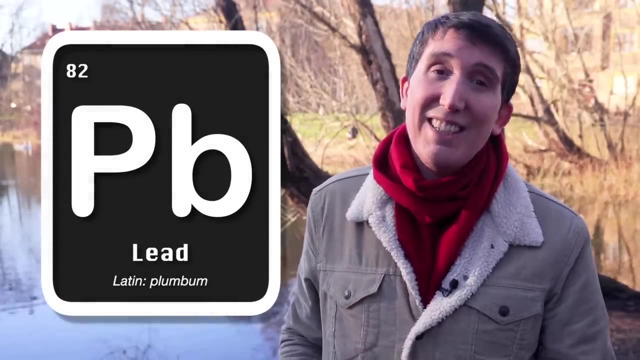 We already talked about mercury, gold and silver. So what about lead? Well, lead gets its chemical symbol from the Latin for lead, Plumbum. We get our word plumber from the same root, because water pipes were often made of lead. 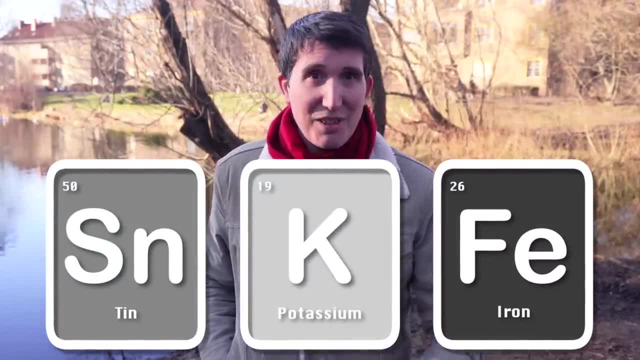 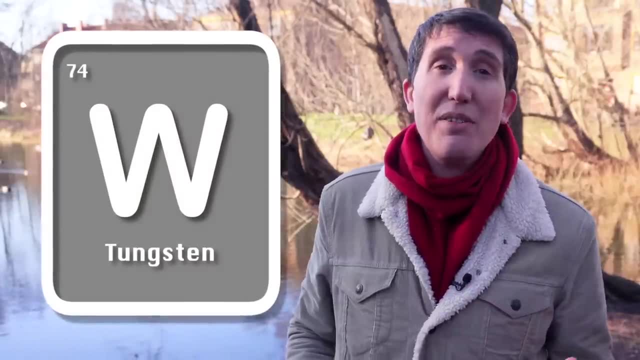 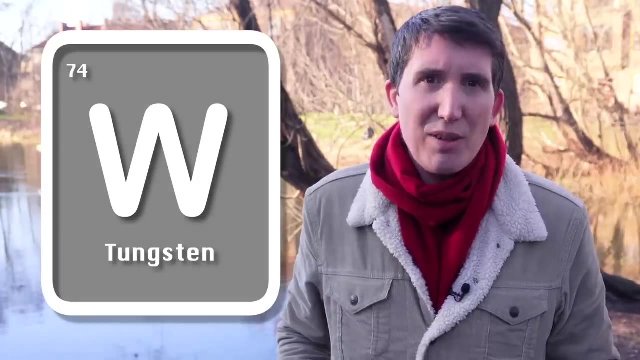 Tin, potassium and iron also get their apparently nonsensical chemical symbols from Latin names for the same metals, And special mention goes to tungsten, which has the chemical symbol W. Tungsten comes from the Swedish for heavy stone, Simple and descriptive.